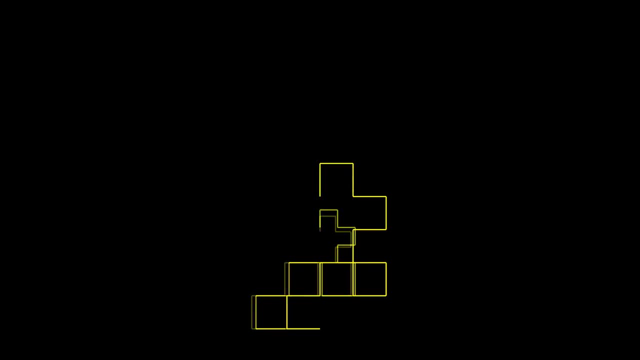 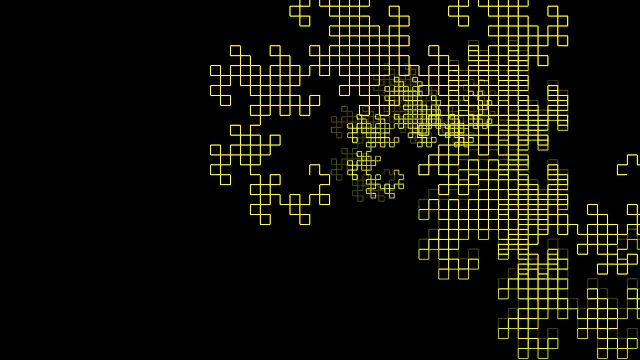 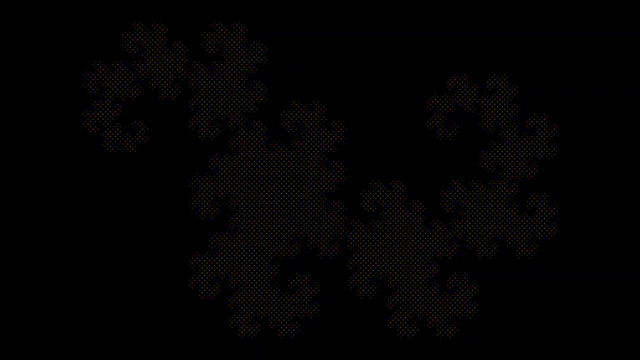 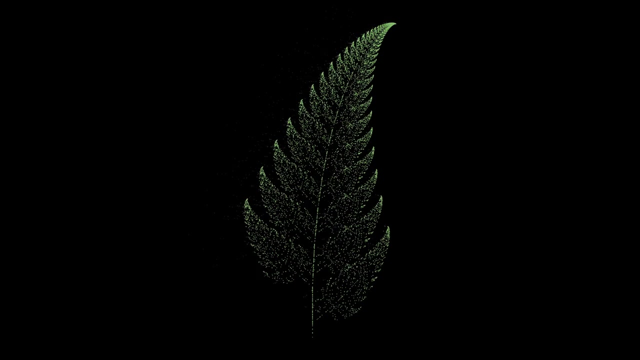 And here's a dragon curve. With each step, the entire tail is sculpted and rotated 90 degrees. The number of parts grows exponentially. Next, look at one of the very natural fractals. This fern was carefully grown by mathematician Michael Barnsley. 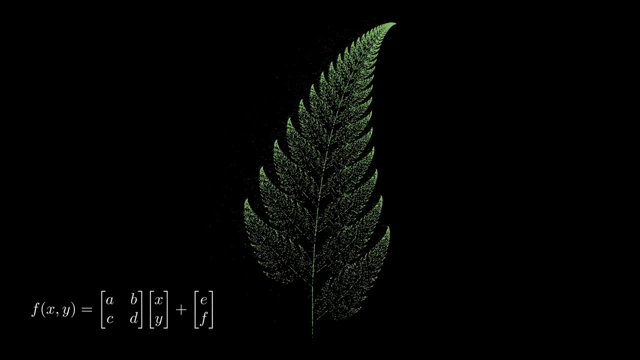 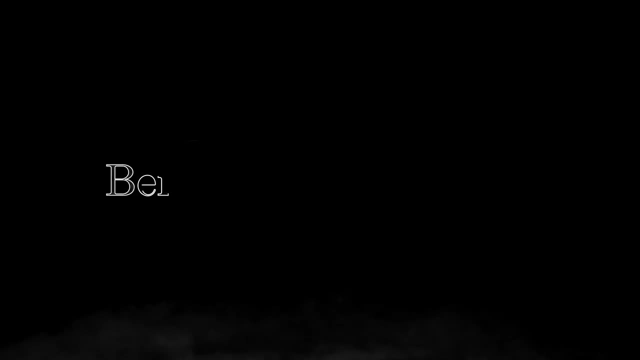 Just one type of FN transformation, and here's an amazing result. Before we will go through more common examples, there is one question about the creator of fractal theory. Benoît Mandelbrot often wrote his name like this: What does the letter B mean? 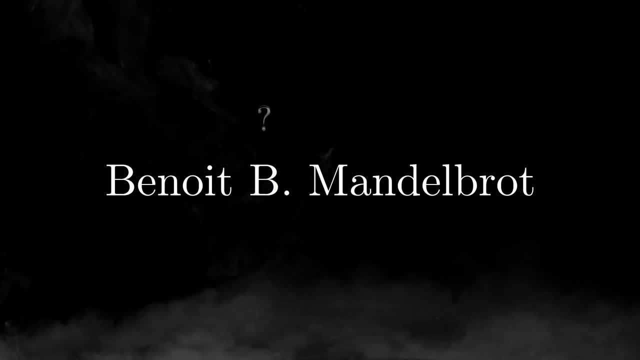 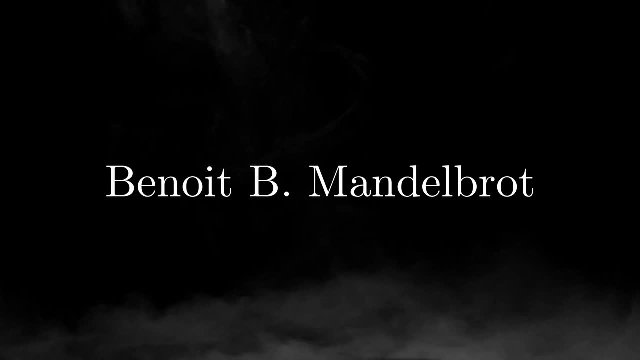 Jesus, You will be given a minute for this question. I suggest that you find an answer within this time span. Also, you can see the right answer at the end of the video. And now for something completely different: The Koch snowflake. 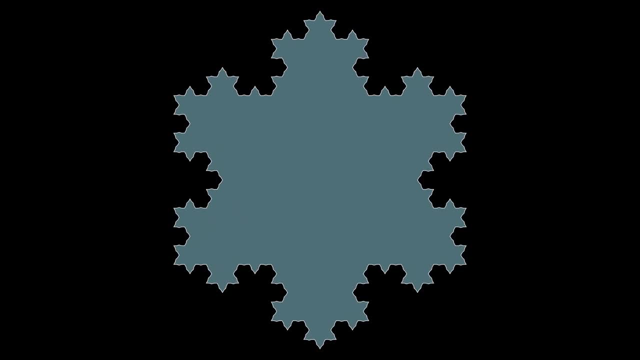 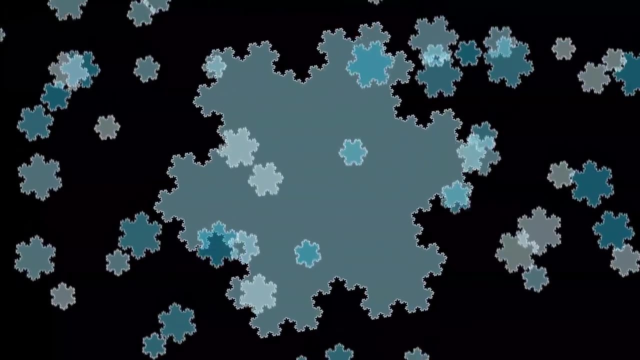 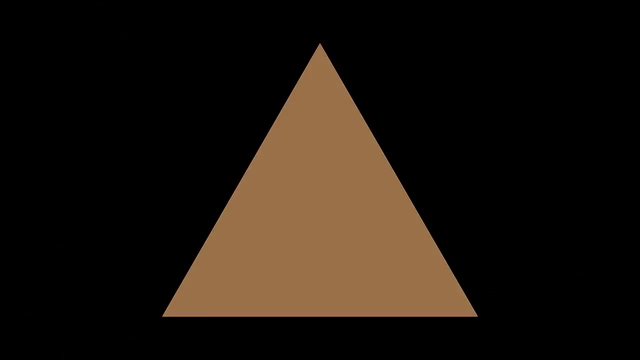 Look how, with every step, the contour is getting more detailed and thin. What will be the perimeter of the snowflake if the side of the original triangle is equal to 1?? The Sierpinski triangle. Here, at each iteration center, triangles are removed. 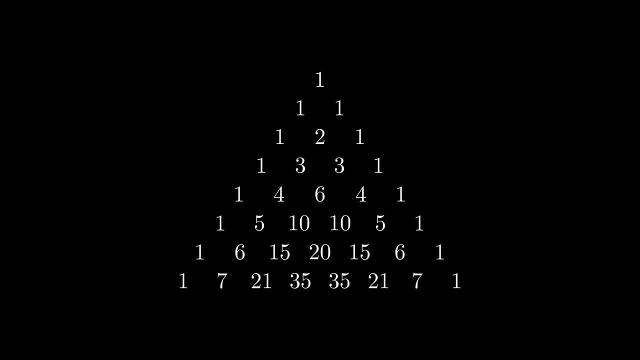 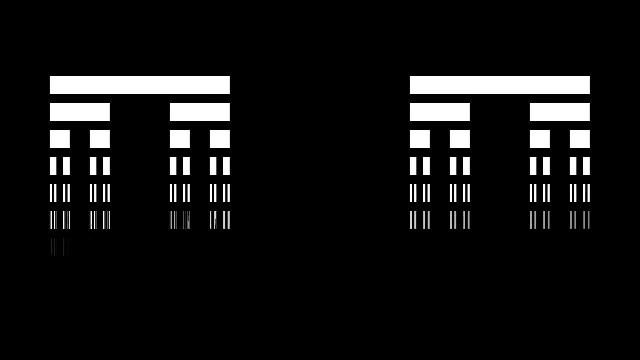 Interestingly, it can also be obtained if we consider the numbers from Pascal's triangle modulo 2.. The Canté set at the end of the 19th century served as an answer to a serious problem of Nowadain's set. The only consensus is that it represents the form of the shape of a new rectangle. 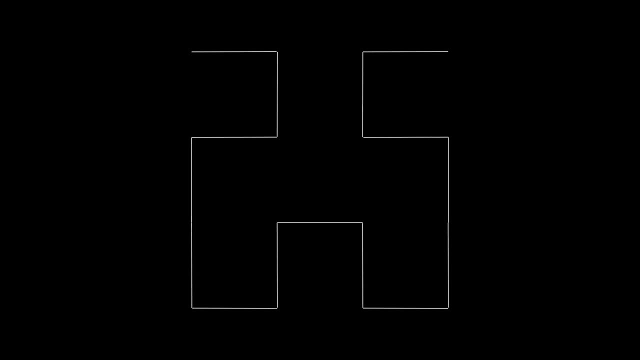 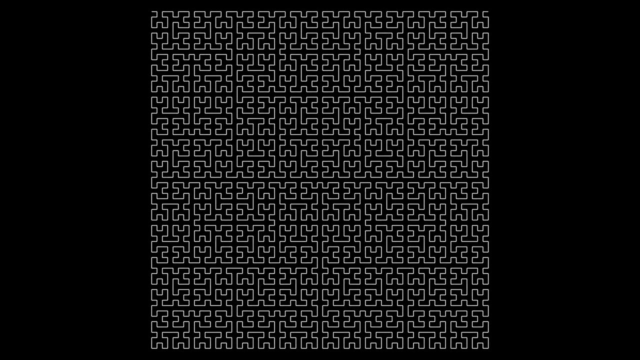 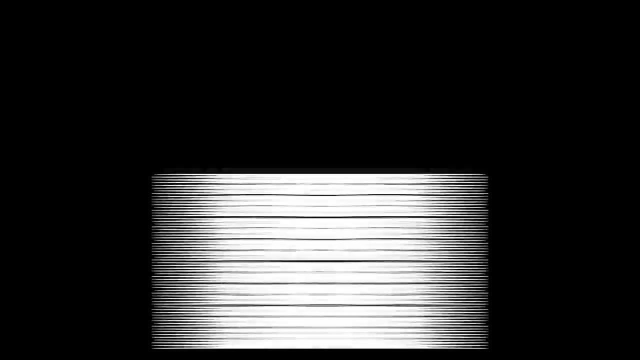 TheJoe Wichner convent. The Hildebrand curve is built in an unusual way. Try to find a pattern of how it is recursively created, starting with a U-shaped polyline. This fractal has received practical application because it successfully maps a segment to a square. 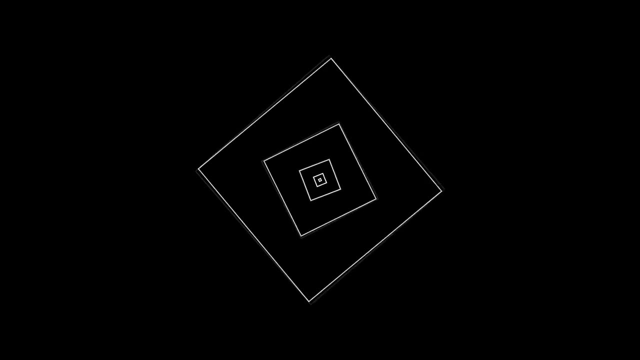 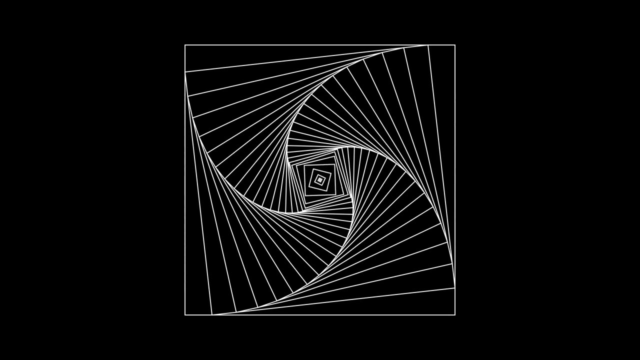 Letters. Beautiful Legavishnik spirals are obtained by recursively applying the connective curves, and so they are more or less identical to each other. recursively applying the rotary homotopy to the square. Someone may notice the ancient Indian proof of the Pythagorean theorem in this construction, and others will recall the wonderful work of the.